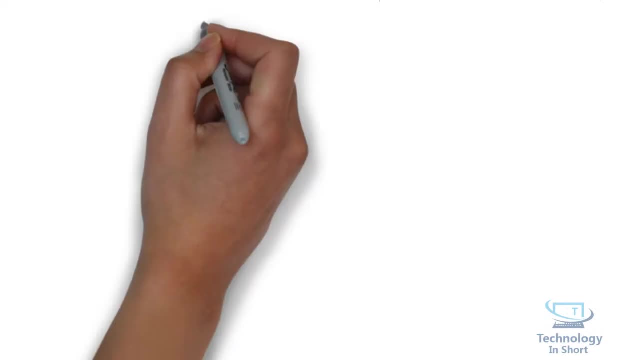 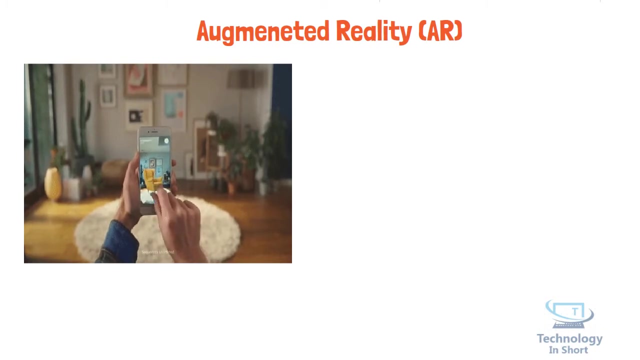 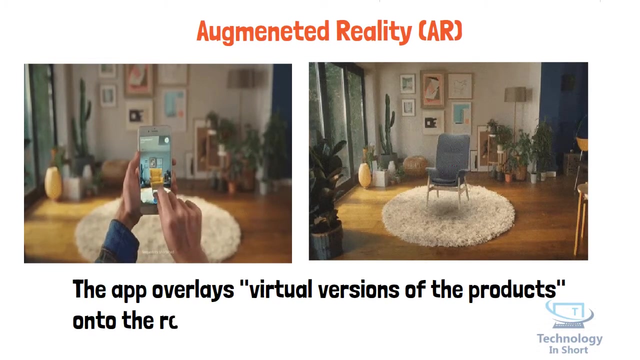 Today we will make it clear. First, let's understand what is augmented reality. Retailer Ikea created an application that helps shoppers to visualize how certain product will look like in their home before they purchase them. The app overlays virtual version of the product onto the real-life images of customer living space so customer can have a look how it is. 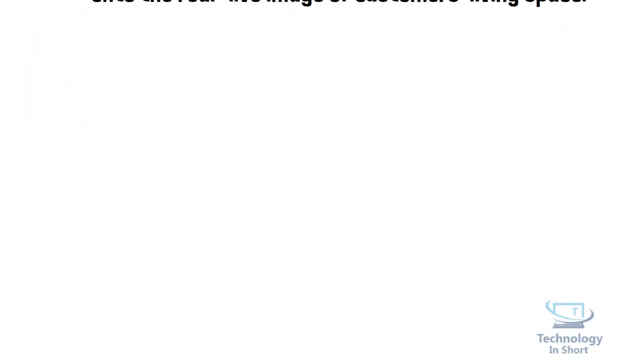 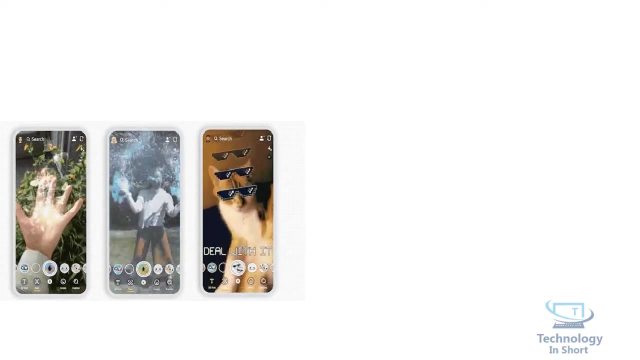 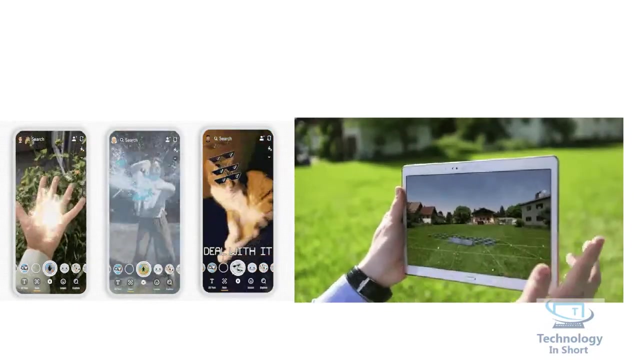 suitable to their home. Also, you all are well known about Snapchat application. In Snapchat, you can add digital content such as additional noise, ears, text and 3D images on your real-time images. These two are just example of AR applications. We can say in augmented 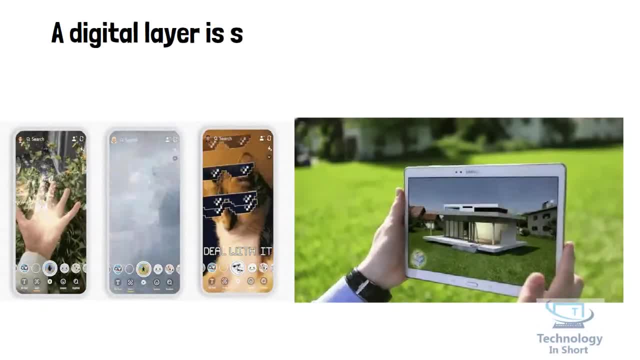 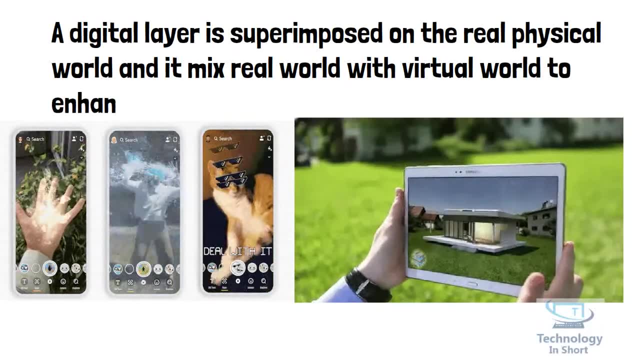 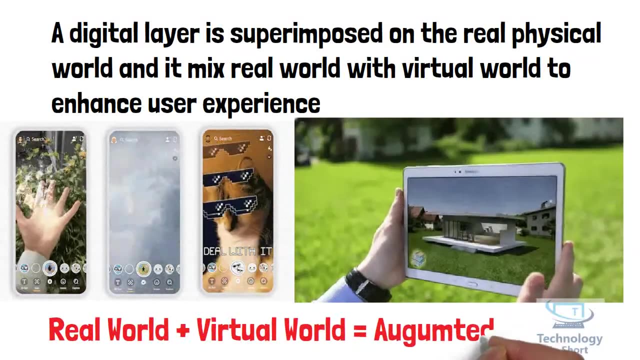 reality application, a digital layer is superimposed on the real physical world and it mixes real-world with virtual world to enhance user experience. In short, we can say that real world plus virtual world is augmented reality. Now let us discuss what is virtual reality. 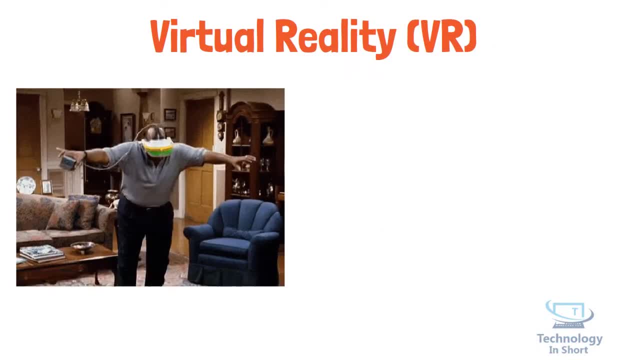 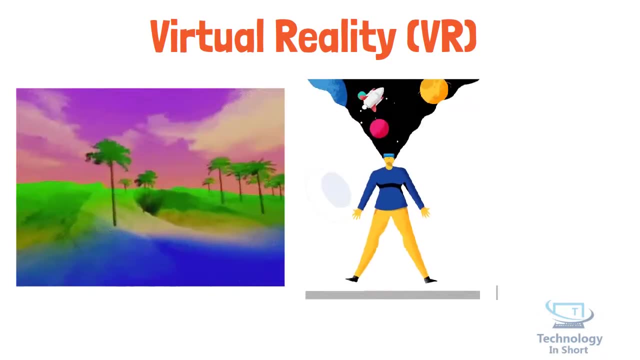 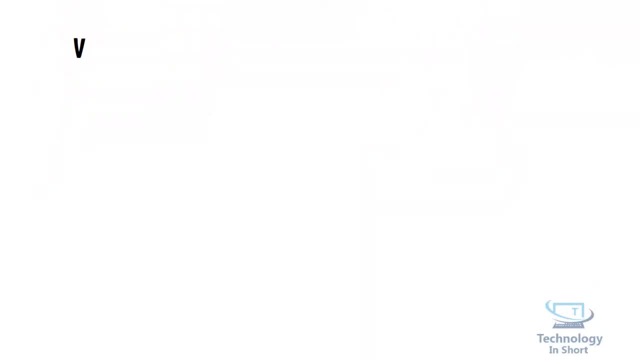 Just imagine if you want to feel like you are walking on the hillside moon or you are swimming under sea. using VR applications you can move to enter virtual world and you can feel like you exist in that virtual world. in short, we can define: virtual reality is the use of computer technology to create. 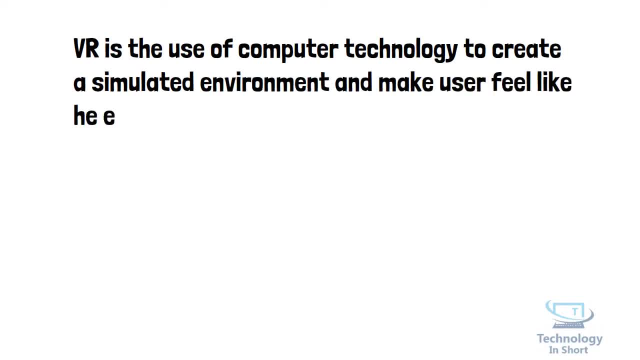 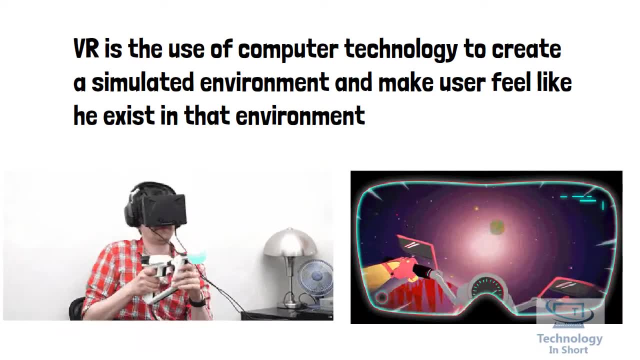 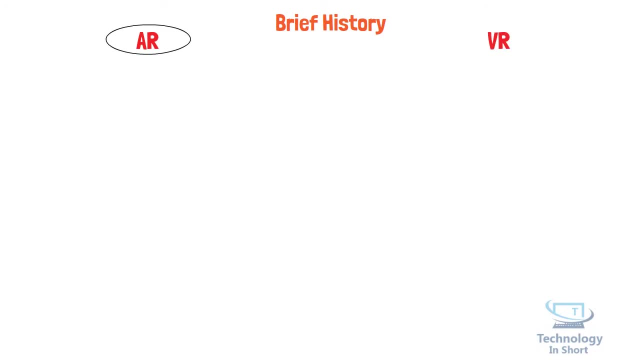 a simulated environment and make you feel like you exist in that environment. it is done by simulating as many senses as possible, such as vision, hearing, touch, vibration, even smell. now let us see brief history of augmented reality and virtual reality. in 1968, a Harvard professor and computer scientist, mr 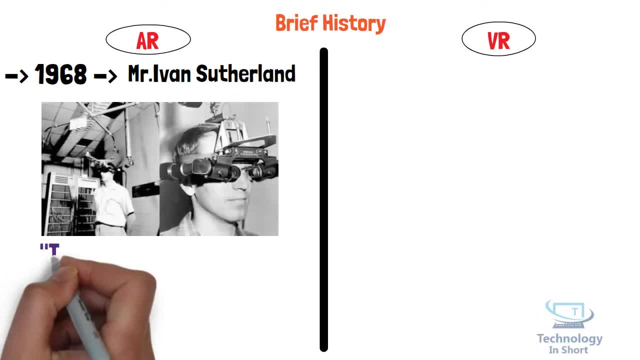 Ivan Sutherland created first head-mounted display called the sword of Damocles. with his device, a user experienced computer generated graphics that enhanced their sensory perception of the world. in 1990 a boeing researcher, mr Tom Caudill, first called it the sword of Damocles. 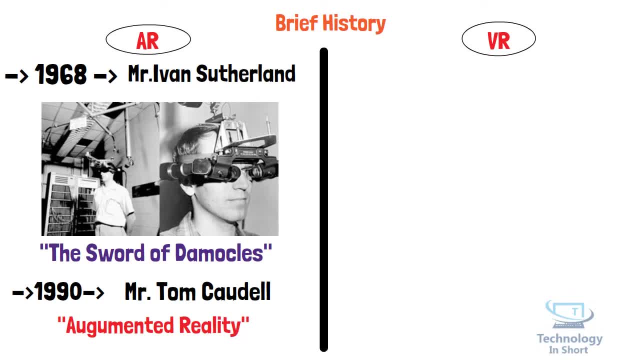 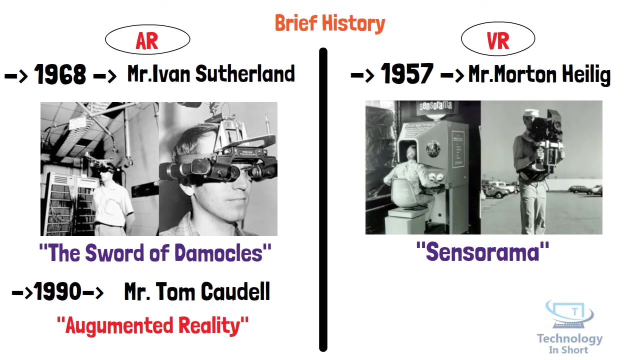 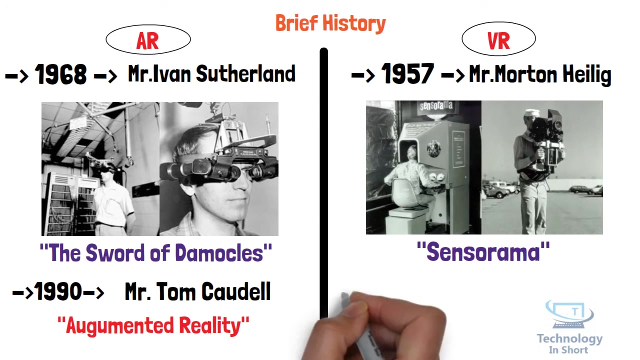 and its well known as the second world war. it was first created in the 1950s by Mr David Hale, who coined the term augmented reality. let us see brief history of virtual reality. in 1957 virtual reality was first achieved to wind. later, in 1987, a computer scientist, researcher and artist, mr john lanier, first time coined the 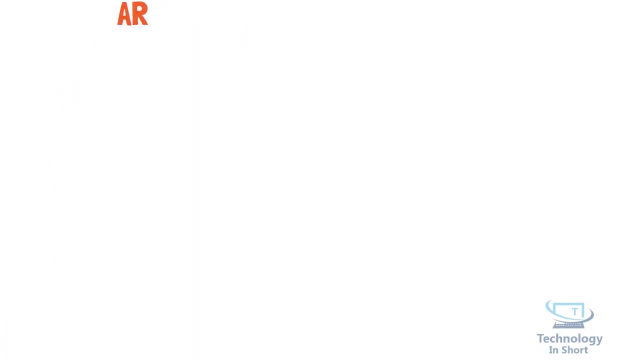 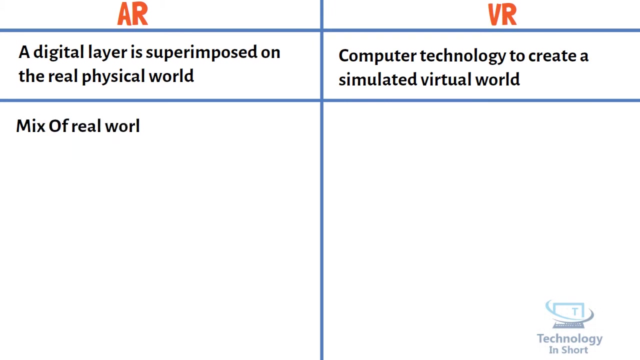 term virtual reality. now let us summarize the difference between augmented reality and virtual reality. in augmented reality, a digital layer is superimposed on the real physical world. in virtual reality, computer technology is used to create a simulated virtual world. in ar it is a mix of real world and virtual world. in vr it creates under virtual world. in ar a user can clearly 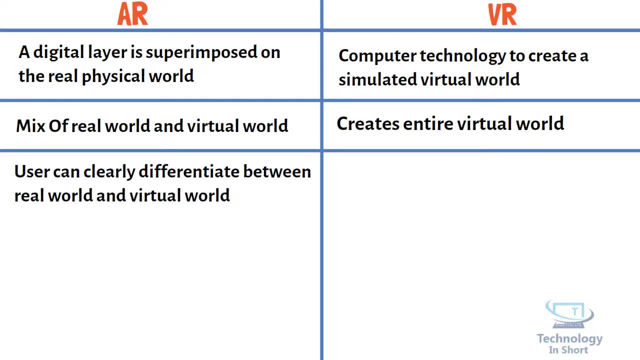 differentiate between real world and virtual world in vr. for a user it is hard to differentiate what is real and what is virtual. in ar, user is not cut off from the real world. in vr, user is completely immersed in artificial world. he is cut off from the real world. 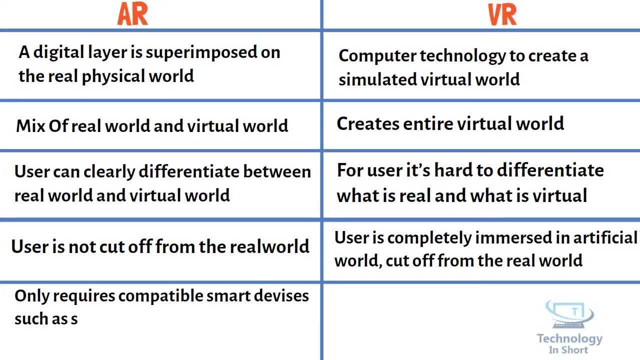 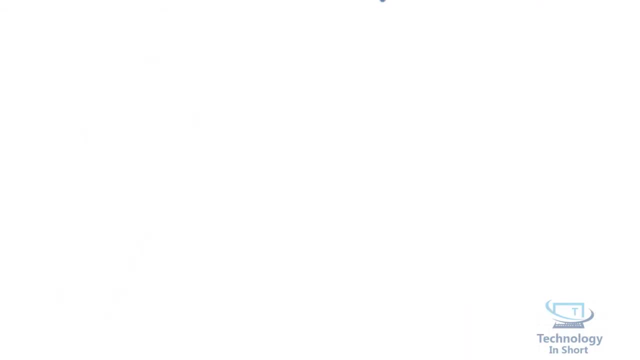 in ar, it only require ar compatible smart devices such as smartphone, tablet, laptop, smart lenses, etc. in vr, it requires head-mounted devices or additional equipments to get fully immersed in virtual experience. these are the basic difference between augmented reality and virtual reality. finally, let us discuss few application of ar and vr. first application is healthcare industry. 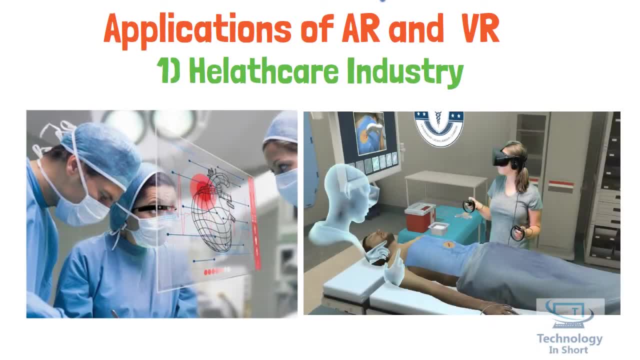 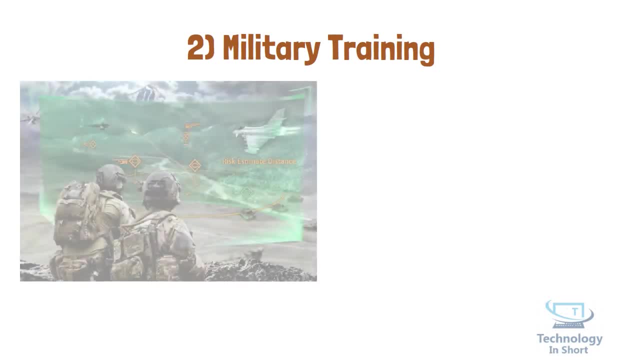 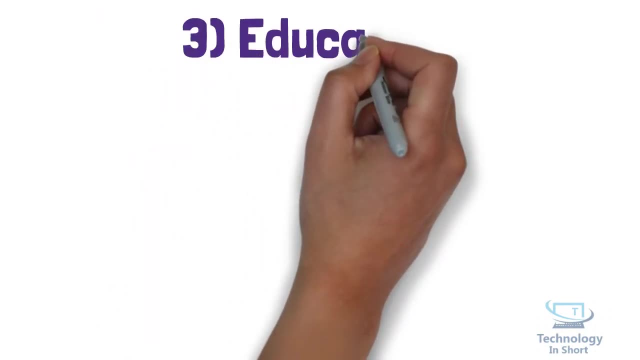 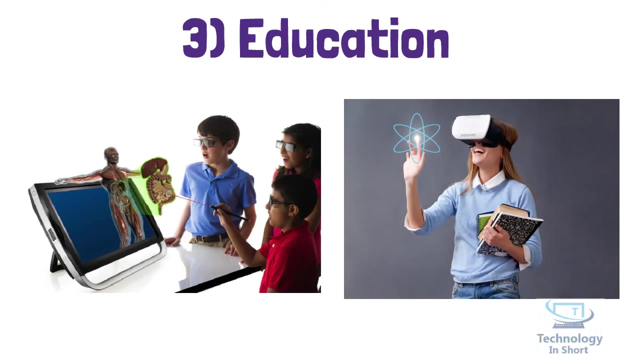 these two technologies are commonly used in healthcare industry by doctors and medical technicians. second application is military training. these technologies are used for military training in virtual environment and creating virtual works. third application is education. augmented reality and virtual reality is used for education purpose. it will give better understanding for students. fourth application is retail and e-commerce.